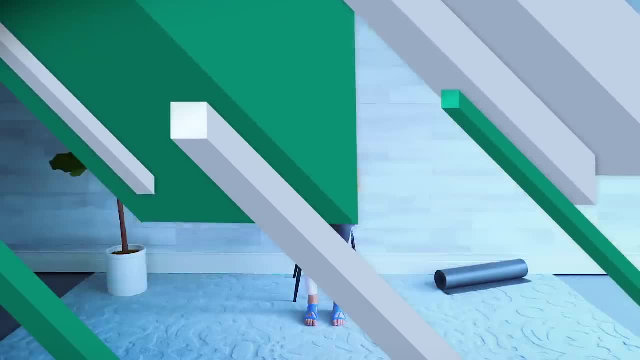 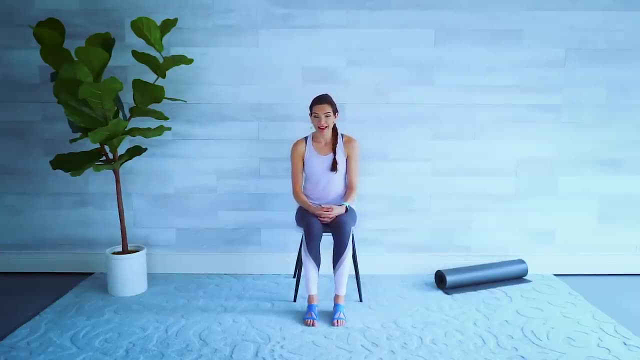 hi, welcome to my channel, senior shape. today I've got a great chair yoga stretch video for you. perfect for anybody, anytime, but especially great for seniors or beginners, anyone that has any joint issues, pain or arthritis as well. we're gonna spend the whole time in our chair, you don't need any. 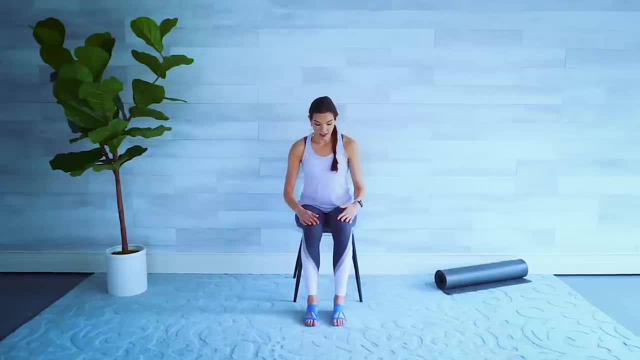 equipment, not even any footwear. I'm wearing today, however, Barlettox little shoes that are perfect for yoga Pilates. they use them for my barre classes as well. they support the foot, but also give you a great non-slip finish, and I love being able to grip with my toes. so I will put the link. 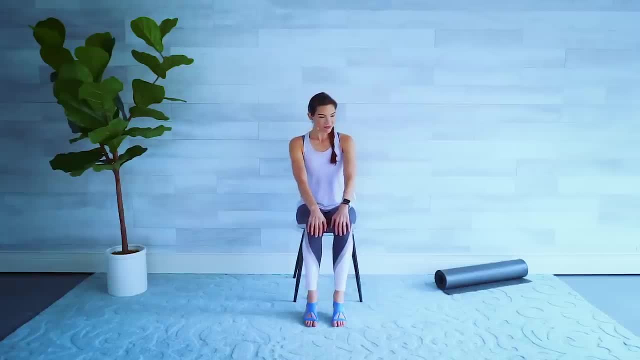 to that in the description of this video. you can check them out, sitting up nice and tall. let's go around our feet, pretend that we have a string lifting the top of our heads, close your eyes, rest your hands on top of your thighs. take a big, deep inhale. 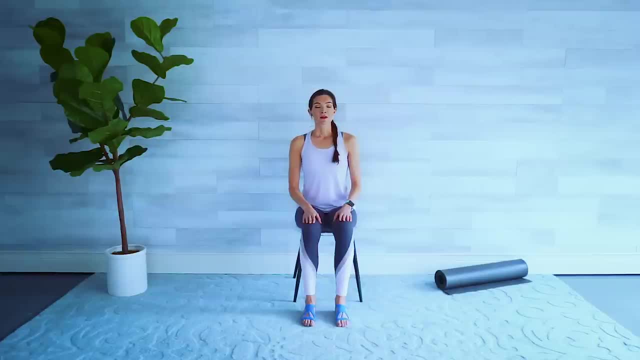 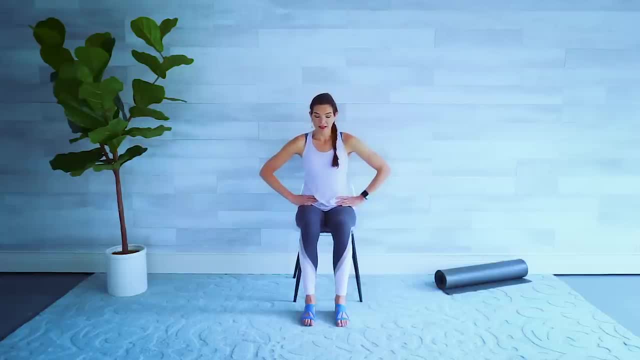 pulling your belly button into your spine, go ahead and round your back slightly, and I want you to tilt your pelvis forward and then release it back, so it's like a little tummy tuck. here we're warming up the core, tilt the pelvis like you're squeezing your glutes together and slowly release tilt. 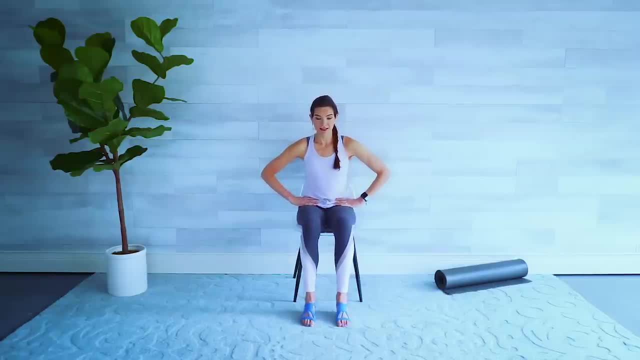 and release just the pelvis. still sitting up, tall shoulders down and back, two more. let's turn this into a cat cow: hands on top of the thighs round the back. let the hands just naturally move forward and back on top of the thighs, pull the belly button in. sit up nice and tall. 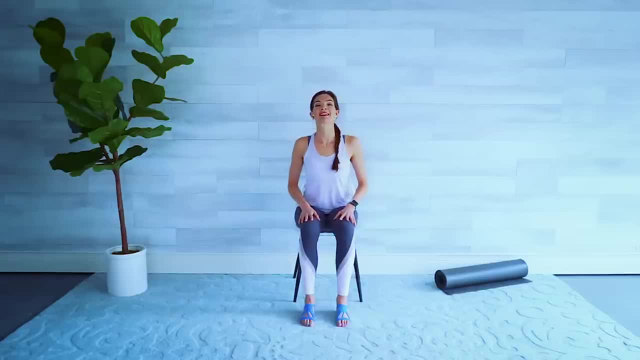 shoulders down and back. nice, just sit up and Mountain Beautiful harder. 197 inhale exhale, inhale, out, exhale, inhale, exhale, up, breathe in. inhale, exhale, out, exhale, inhale, behold, exhale and up, chin, up, chest, proud shoulders back. add again: drop the chin like you're gazing at your belly button, and up, chin, up, chest, proud shoulders back again. drop the chin like you're gazing at your belly button, and up, Let's do two more. 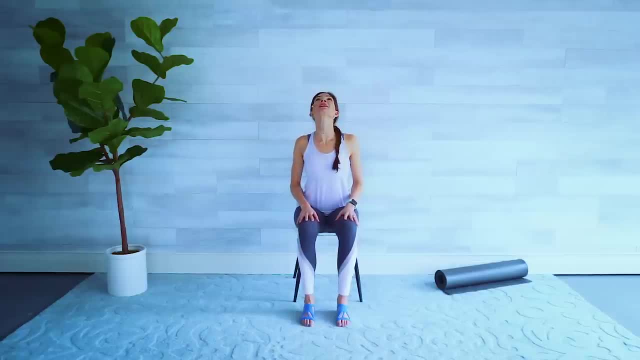 the nice is big, nice and big as we're warming up here. good, find your way back to Center, come to the edge of your chair and separate your feet just a bit. we're gonna do a nice little body roll here. so hands on top of the thighs, and I want you to kind of undulate your torso here leaning. 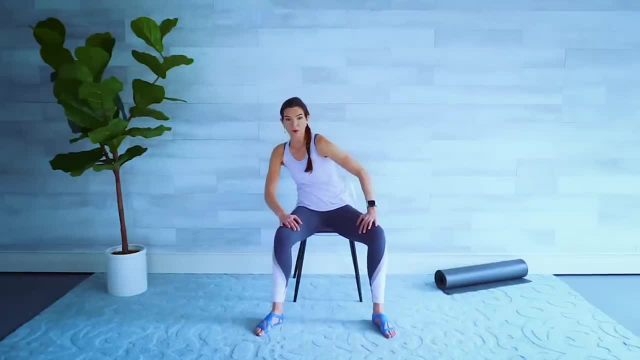 forward and then round the back all the way back. so stay in one direction and you're just drawing a big circle here with your torso round and then chest forward. good, nice and slow. I should feel really good on your back. let's do one more this side. 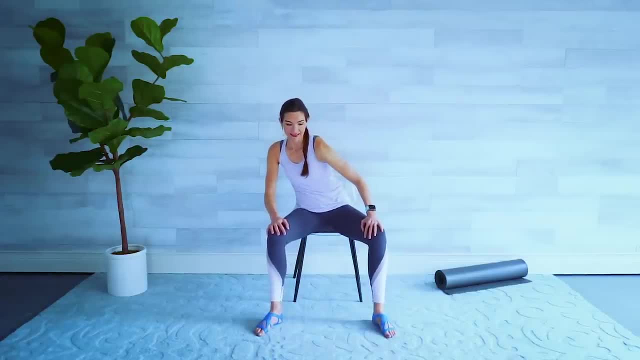 good, find your way back to Center and other side. make sure you go ahead and switch nice deep breaths as we do this, filling it in our core, really warming up the spine and the back of the head, and really warming up the spine and the back of the head and 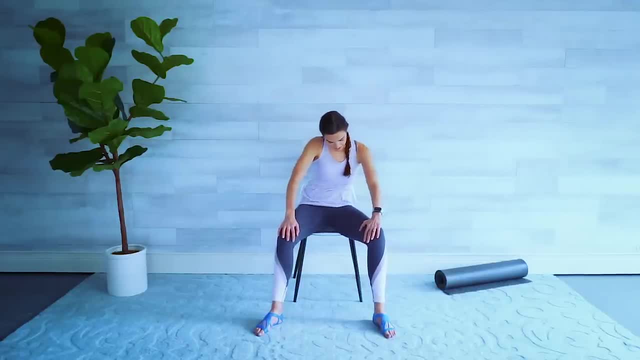 that spine. so one more good toe heel bows feet back in. so their hip with the part making sure the ankles are underneath the knees. go ahead and big, deep breath. arms go up, put those palms together, reaching as high as you can, and then bring it down to prayer here. 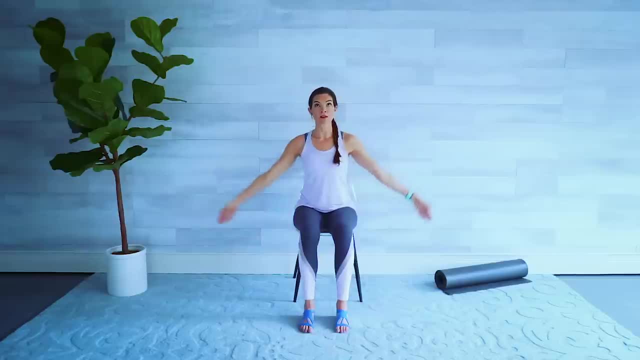 elbow, elbows out to the side again. inhale, reach those arms up, exhale down here. inhale arms go up and down. inhale up big reach, exhale down into prayer. one more: inhale up, exhale down into prayer. I want you to hold your hands here, so thumbs. 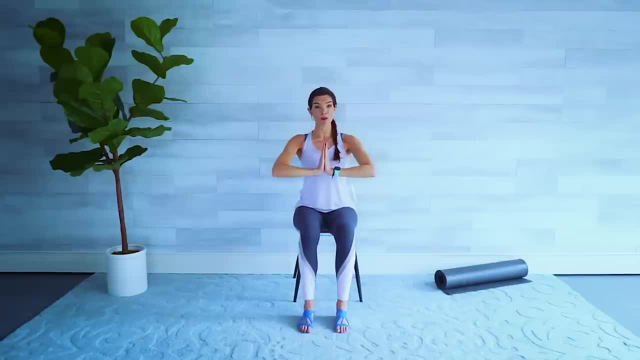 are pretty much at your breastbone. here in between your chest, elbows are out to the side. push those shoulders down and back and I want you to turn your fingertips towards your breastbone, feeling that beautiful stretch in the wrists. come back up and then point your fingers towards me and back to Center. 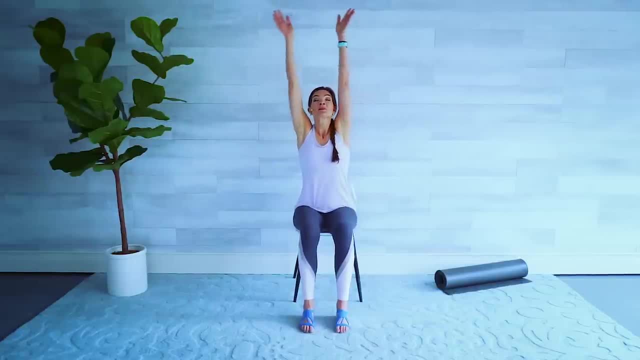 good, let's do that again. inhale, arms, go up, exhale down to prayer. turn your fingers towards you, back to the top, towards me, back to the top one more time. inhale and exhale towards me, feeling it really nice. stretch in the shoulders here, keep the elbows high towards the ceiling. 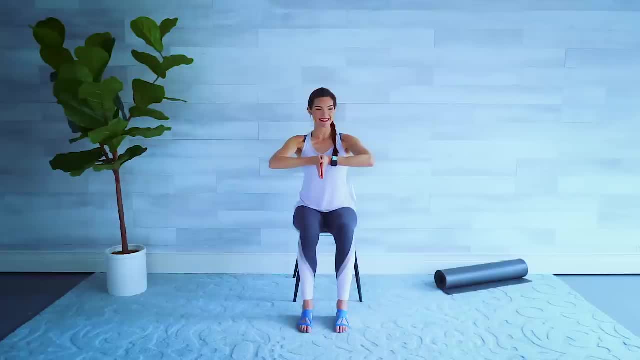 that's very 다시en. all the way to the bottom. inhale after any. Dziękuję here. now move yourственный and then towards me, back to Center, and release it down. reach her right up towards the ceiling as high as you can, and then we've got a big stretch over to the side. 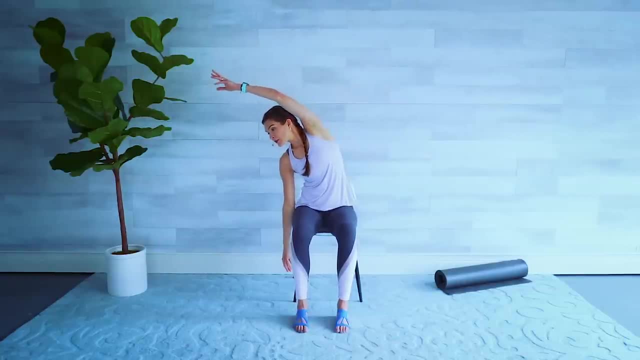 big reach. always keep your core engaged here so you're not using your lower back holding you up as you stretch over one more each side. inhale arms up, exhale over. inhale arm up and exhale over. bring that right arm up again and I want you to cross it over your body. and if 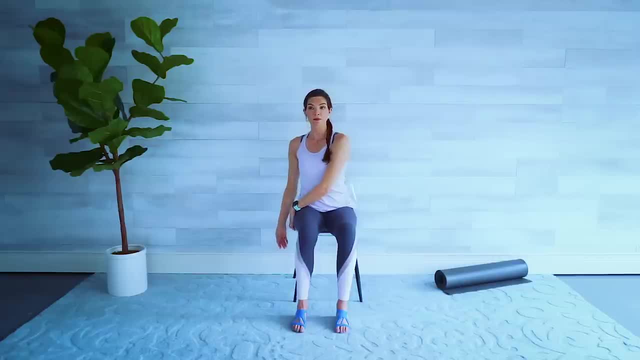 you're able to hold on to the side of your chair. left arm comes up and then hold this nice big reach over here. oh, that feels good. hold, inhale and exhale, release that arm down, uncross. left arm goes up, crossing over the body and holding onto the side. 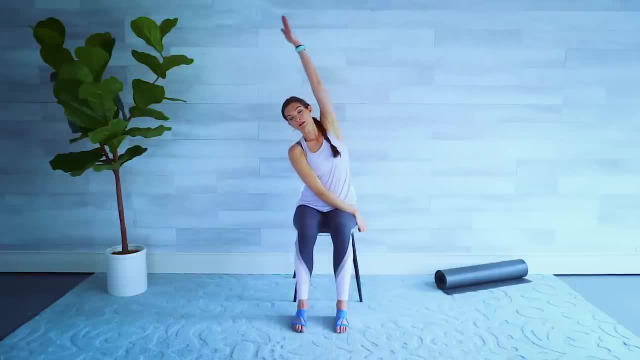 of the chair. right arm reaches up and then a big stretch over as you support yourself, intensifying that stretch in the waistline and all the way up the arm. release it down, uncross big, inhale arms, go up, reach those fingertips towards the ceiling, tummy in then. I want you to hinge forward towards me. 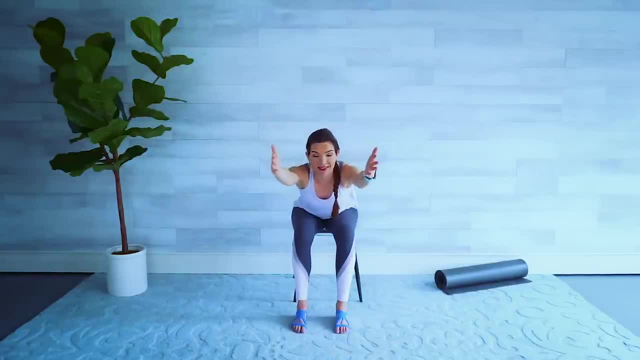 not rounding the back. reach, reach, reach, reach forward. drop your chin just gazing ahead of you. take another big inhale and, on your exhale, go ahead and round your back and drop your hands towards the floor. it's okay if they don't reach round your back, drop your head and do it feels. 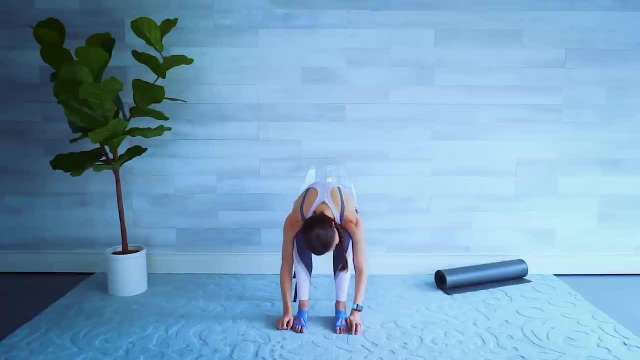 good, right here. maybe you want to shake your head, yes and no, releasing any tension, finding your breath, relaxing all the way from those toes, fingertips and lower back: inhale, exhale, put that tummy in and then let's slowly roll it up, one vertebrae at a time. 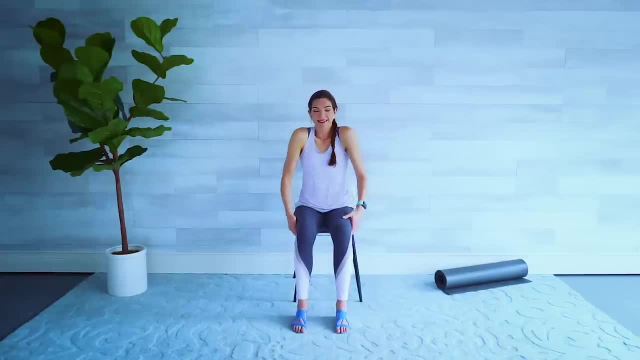 got to follow with the shoulders here. big shoulder rolls open up those legs so you have a nice wide stance here. inhale arms. go up again, fingertips towards the ceiling. now really plant your feet and place your weight in your feet without reaching up out of your chair. reach again towards me, weight in the feet so you don't fall forward. inhale, exhale. 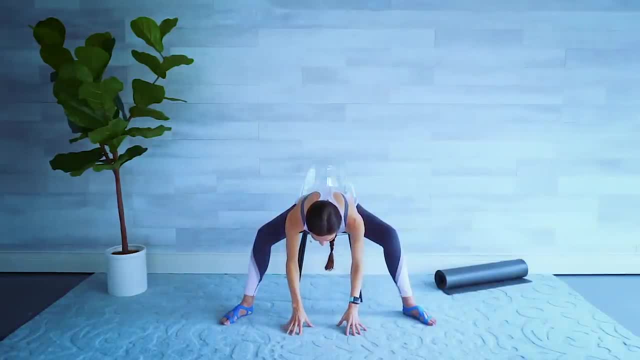 again, drop all the way down, if you can. if you can't come all the way down, you may leave your hands right here on top of your thighs. feel that inner thigh stretch, drop the head, inhale, exhale. if your hands are on the ground, go ahead and move them up to your thighs. 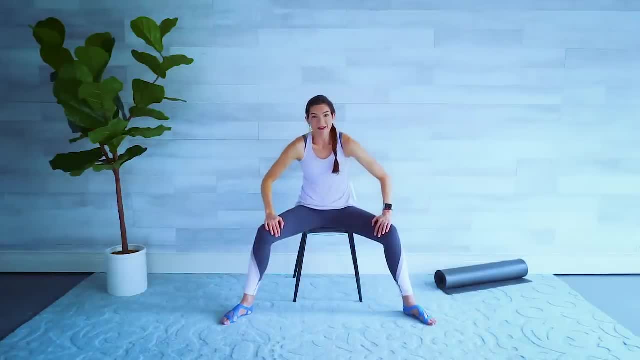 tummy in and let's roll it up nice and slow. good job taking your left elbow. i want you to lean forward all the way from that waistline onto your left leg. let's take your right arm all the way up, if it's comfortable for your neck. 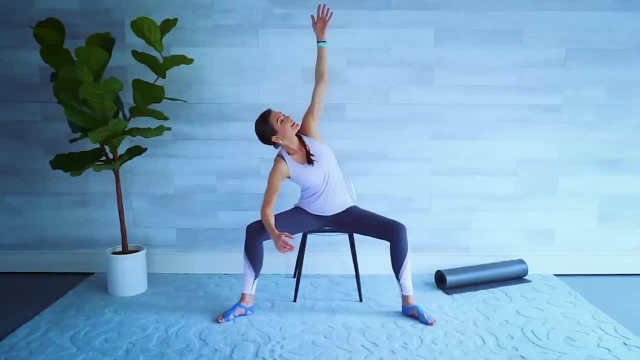 go ahead and gaze up at that hand, feeling a really nice stretch again in that side body, reaching up with those fingertips. inhale here and exhale. if you're comfortable here to intensify this, you can go ahead and drop that left hand towards the floor and go a little bit deeper. 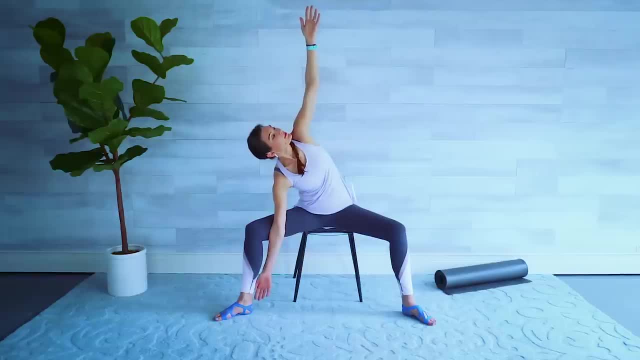 again: inhale and exhale. let's come up, both arms to the side, other side- let's drop that right elbow on top of that right thigh. left arm reaches up and, if you're comfortable, go ahead, gaze up at that hand. big inhale, exhale, stay here or option to drop that lower hand. so this is like a modified triangle position. 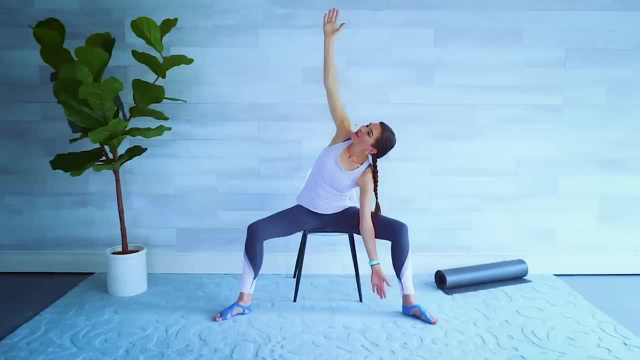 inhale, exhale, inhale. both arms come to the side as we come up. drop those hands and we're going to go ahead and forward. fold one more time, reach those arms towards me, weight in the feet, reach, reach, reach, reach and then go ahead and 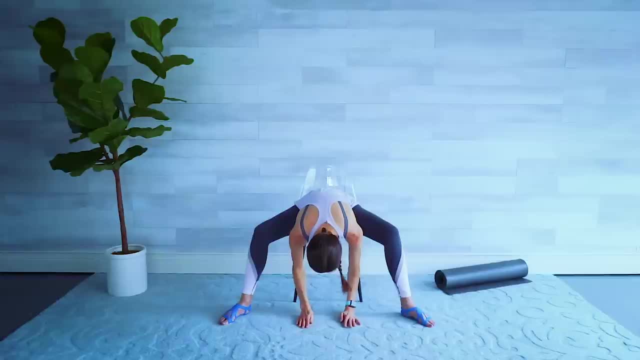 round it down, tummy in and let's roll it up, one vertebrae at a time. hands on those knees. again, i want you to drop your right shoulder to your left knee, feeling a nice twist opposite way. let's do that again. you might feel that in your back and your shoulders. 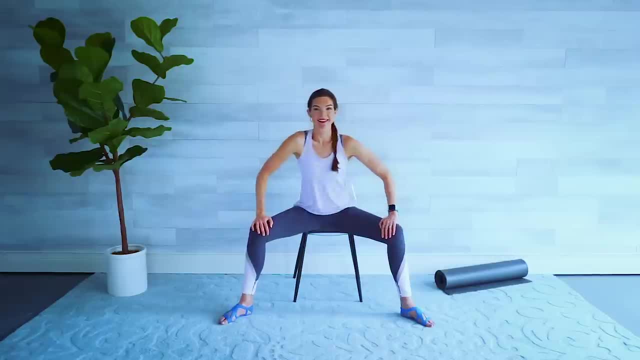 really depending on where your body needs it. it's going to tell you to work on that shoulder. we're going to do it in the front, so we're just going to do that again. last one: let's hold it here. so you're leaning slightly forward, your tummy is in. 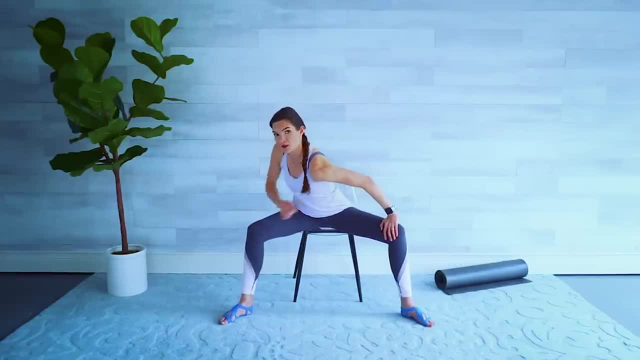 and really emphasize that stretch, bringing that shoulder towards the knee. you should feel it especially right here in front of the shoulder. come back up to seated and let's hold the other side shoulder, dropping down at that angle, and let's come up. excellent job, we're gonna turn all the way to the side in our chair scooching. 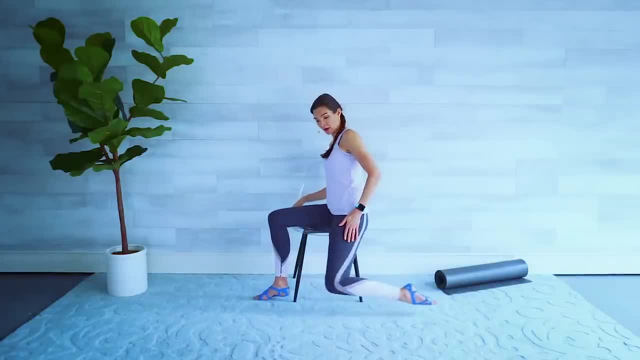 back here. this outside leg is going to come down, so as if, like we were kneeling, but the knee is not going to touch the floor. front leg is bent at a 90-degree angle, and then go ahead and stretch that back leg out or front leg out as much as you can for a beautiful hip flexor. 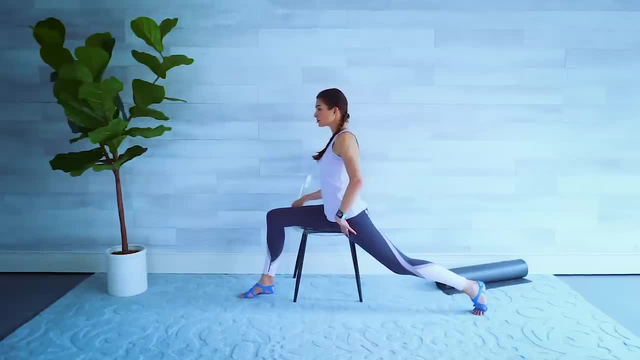 stretch here. so sitting up, nice and tall, think about doing a little pelvic tuck here to feel that hip flexor. let's inhale as our arm comes up- same arm as leg extended- and exhale as we bend over towards the back of our chair to emphasize that stretch. 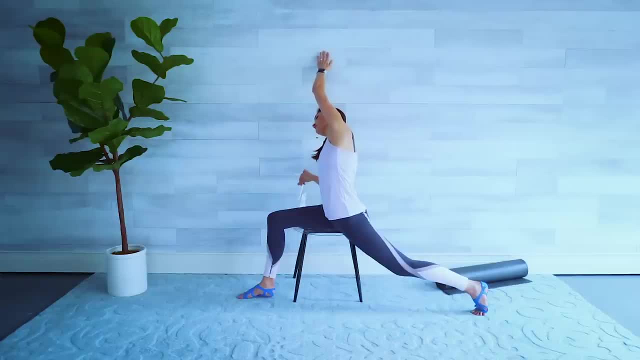 release that arm down. I want you to go ahead and open up both arms here towards the front and then turn that foot so the toes are facing me and then here to the side. so here we are in a warrior pose. go ahead and gaze over that arm in the direction that your knee is pointing. 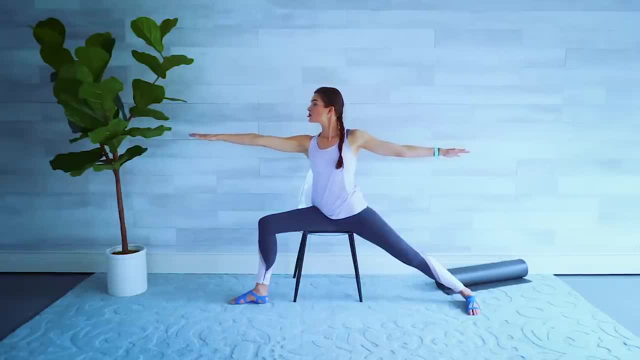 nice and tall. think about your posture. shoulders are down and back, opening up the hips holding this warrior. if you'd like a little challenge today, optional, but I challenge you to go ahead and lift that seat out of the chair, to emphasize that pose: inhale, exhale and let's release it down. 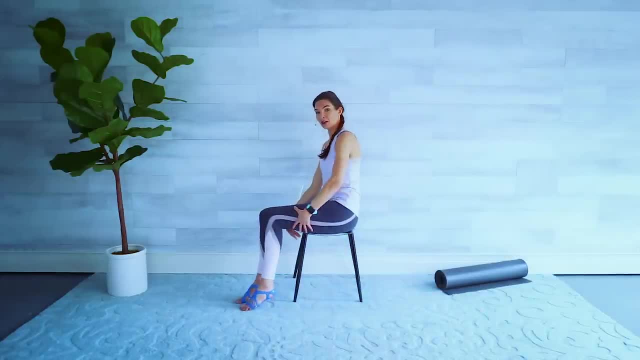 go ahead and bring that back foot to the other knee, drop the hands, let's swivel to the other side. so, starting with that hip flexor stretch, we drop that knee, curl the toes towards the floor, stabilize this front foot toes facing the side and then extend that back leg again. what we're 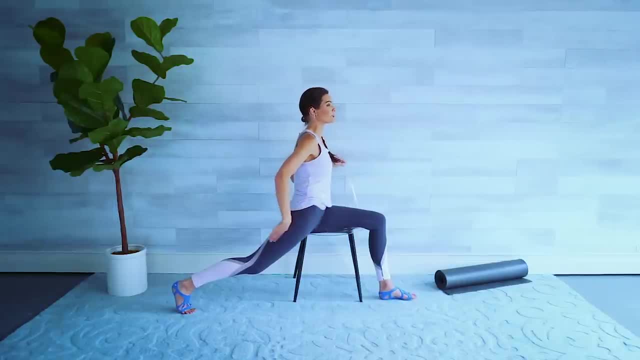 going for. here is the hip flexor stretch right here which is usually so tight from sitting all day: arm inhale, reach up, straighten the back knee. if you can exhale over and lift back up. let's release those arms to the sides here. turn that back toe, so foot is. 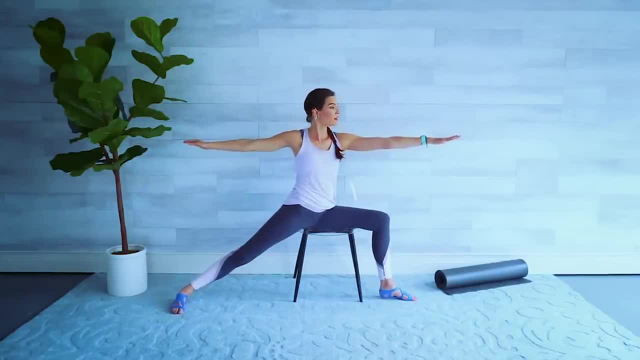 flat on the ground, toes pointed towards me. now go ahead and gaze over your other arm following your knee. make sure you're breathing again. option here: if you'd like to go ahead and try to stand up into that warrior pose, reach those fingertips as far as you can away from. 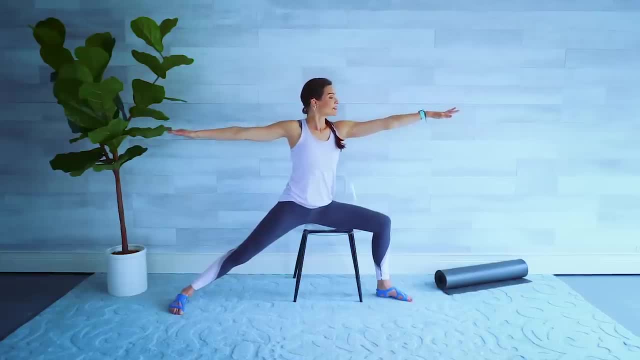 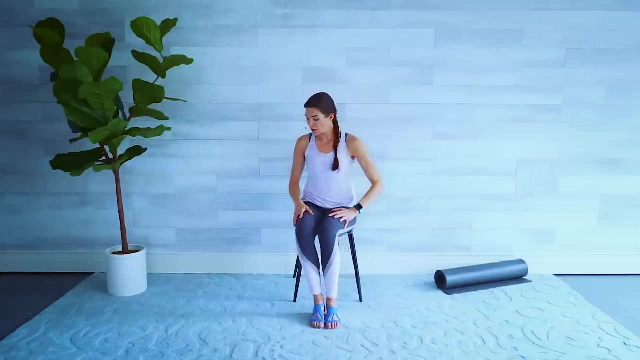 each other. inhale, exhale. sit back down, release the arms. let's bring that other leg forward and go ahead and twist back towards me. excellent, without doing the hip flexor one more time, we're gonna go back into that. warrior, extending that leg should feel a little better this time. arms go out, palms down, gazing over that hand. 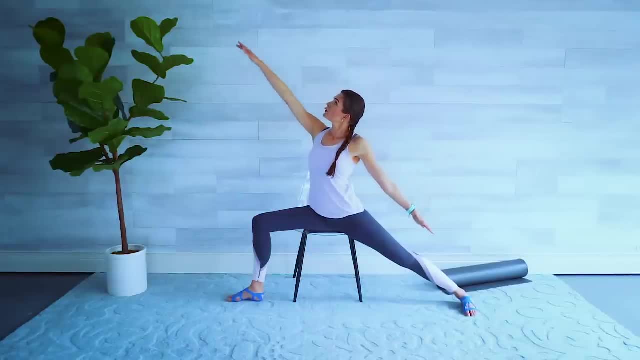 inhale. we're gonna one meal our arms here reaching up, feeling that beautiful stretch and other way you can rest your elbow and stretch over. let's do that again. one mil up here, exhale over. let's go ahead and switch that ftir moving that leg and let's try one more time. 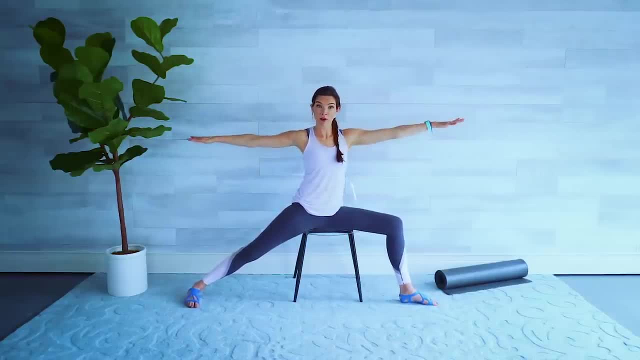 and we're gonna stretch that leg up, slowly extending that leg toes towards me, feeling your hips open up, palms down, gazing over the other hand, reach it up and back and all the way over again, all the way up and back. just a little stretch in the back there, guys, don't push this. 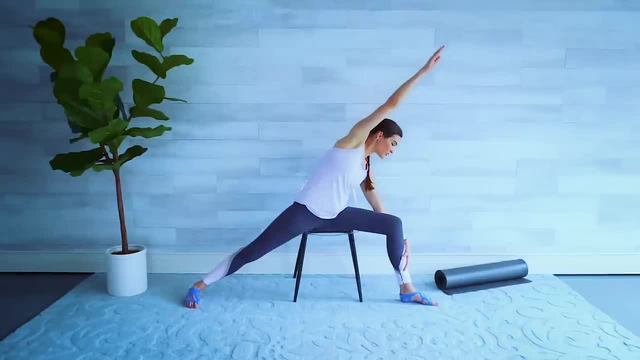 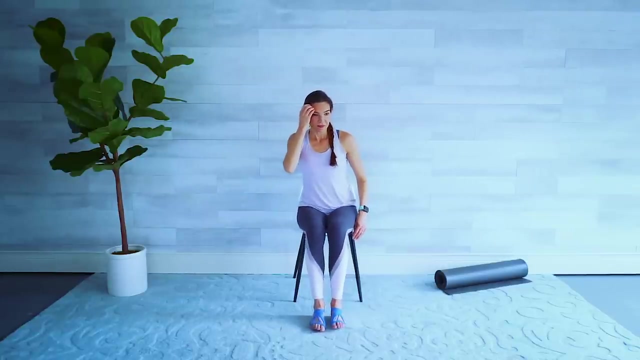 and over big reach, release it, drop the arms and then come back to Center. nice job. sitting to the edge of your chair, extend your right leg out, try to straighten the knee. heel to the floor, toes to the ceiling. arms. go up, big inhale and let's. 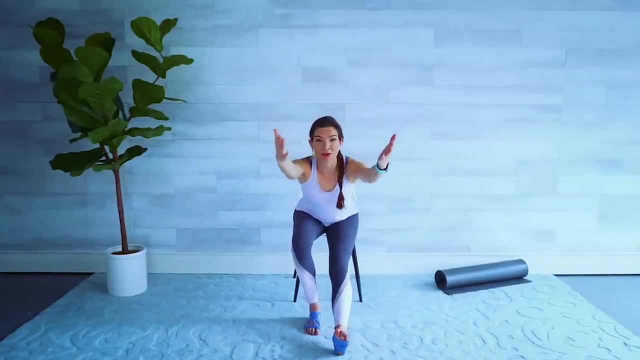 exhale. reach towards me, keeping that spine neutral. hold it there. inhale. exhale round the back and come all the way over. inhale, exhale, tummy in and roll it up one vertebrae at a time. leave that leg there big. inhale back into that prayer position, hands together. 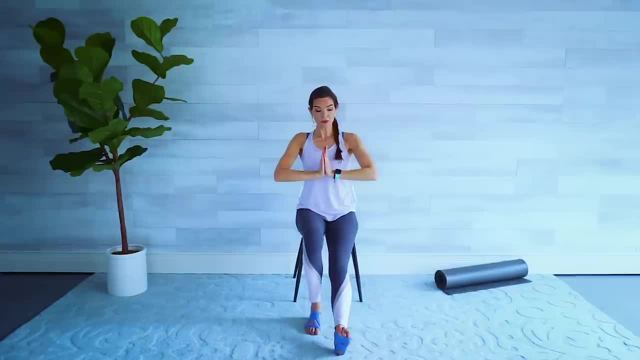 elbows out to the side, holding the leg there. I want you to twist, bending over trying to get that upper elbow back behind you. so you're trying to get elbow towards that knee. let's come up and other side. so again, elbow to the other knee. inhale, exhale, back to Center. really sit down, bring that right leg in left leg. 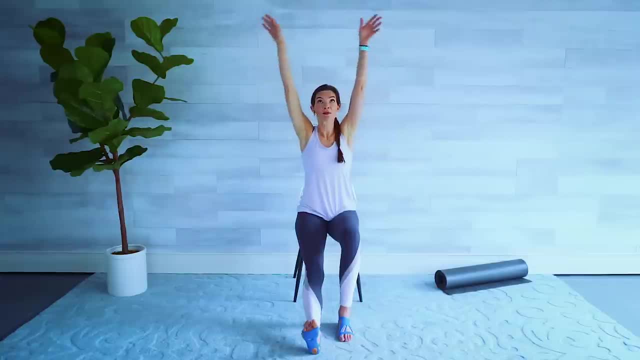 goes out again. inhale up, reach their arms towards the ceiling, reach towards me, feeling that stretch all the way up the back of the leg and that hamstring. inhale, exhale round forward, fold, breathe in, breathe out as you roll up one vertebrae at a time. leave the leg. 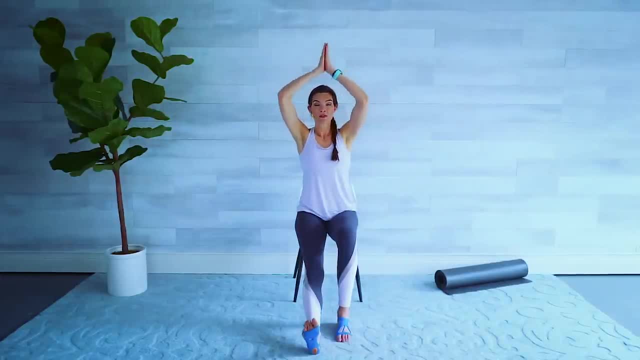 there. inhale up. yes, come to prayer. elbows to the side. here we go again, hinging slightly forward elbow towards that straight knee you burn to circle one and avoiding being σ up back to center. other side. inhale, exhale 3-4-3 and up. 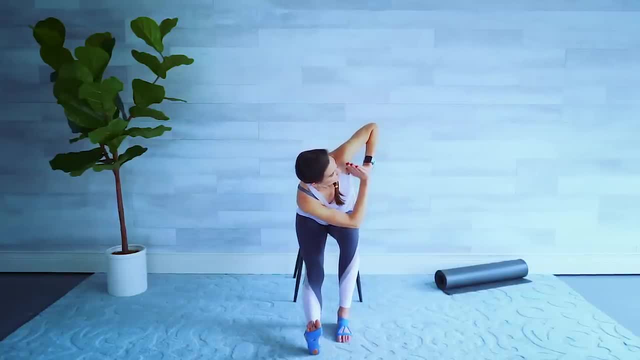 inhale. last onecią confronted: oppose Ei, turn and roll up. tuck your foot, placing, say, to the right and back to center. go ahead and straighten both legs, making sure that you're firmly on your chair. arms go up. inhale, exhale forward. 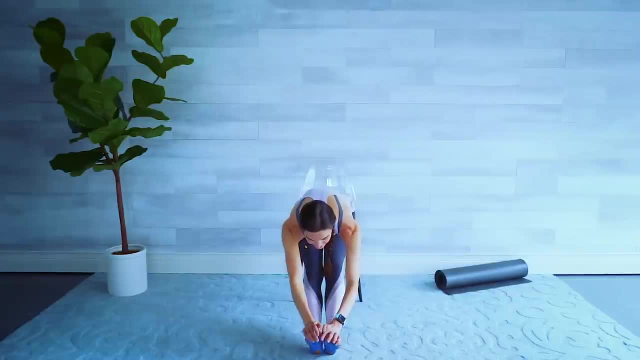 hacia la elefanta. fold over both of those legs. Düntare vega can't no big deal as long as you're feeling that stretch in the back of the legs. big inhale, exhale. can you go one more inch? let's go ahead and roll it up, letting your arms guide you here all the way. 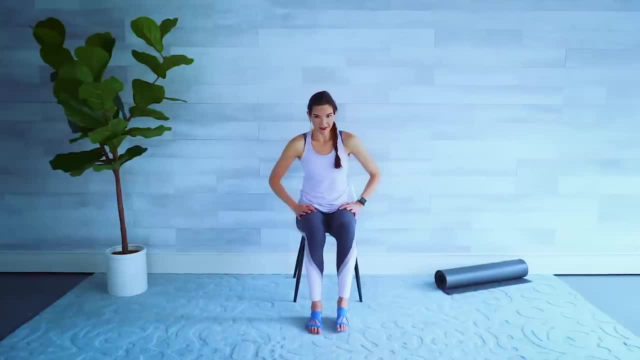 up your legs and go ahead and bring those feet in sitting up nice and tall, separate those legs again. arms go up overhead, palms facing each other parallel. and then i want you to do a little cactus here, elbows out to the side and bring those shoulder blades down and back behind you. 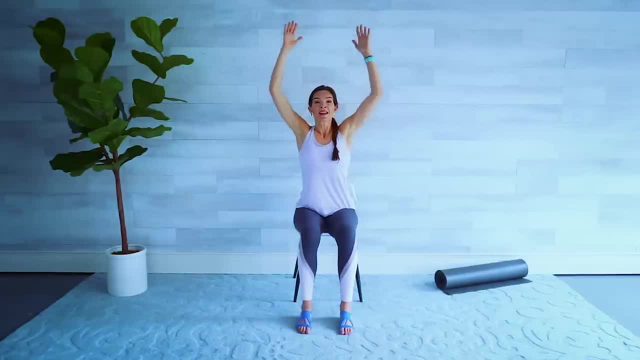 good. inhale up, reach it as high as you can. exhale, open up that chest. inhale up, exhale one more time up, exhale down, keeping those elbows bent. go ahead and cross that left arm over the right, squeezing the chest into a little eagle position here, if you're able to, pressing your palms together. 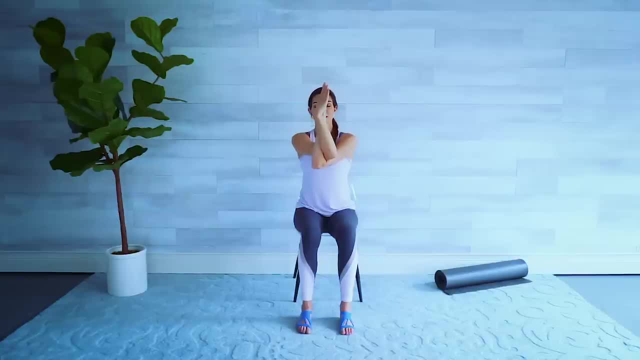 sit up nice and tall to emphasize the stretch. let's pick up those elbows, lifting those hands- exhale, let it drop back down. let's do that again. inhale up. we're going to do a little bit more of that: exhale, exhale lower and let's uncross, reaching back up top. inhale, exhale, cactus, inhale up. 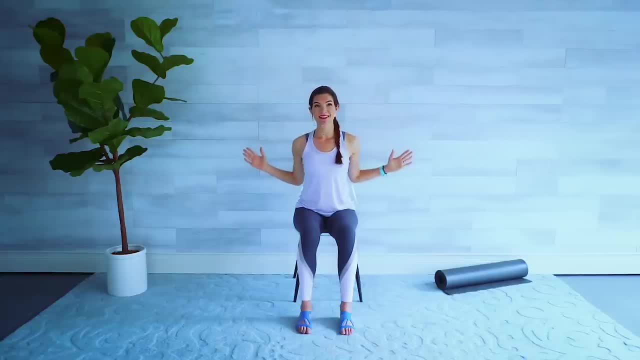 exhale. squeeze those shoulder blades behind you, inhale up, exhale down. one more elbows back out to the sides this time. cross the other arm on top right arm on top of the left, twist those hands around, push those palms together. shoulder blades are down and back. 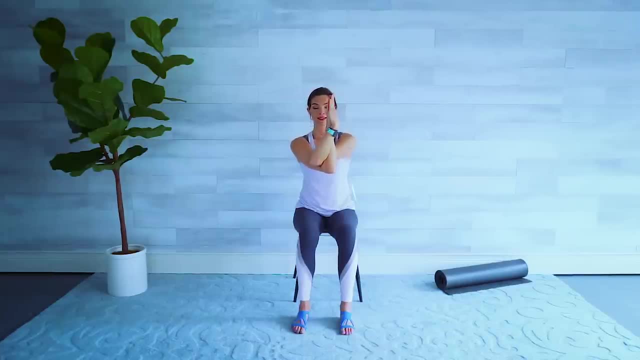 inhale. lift those hands up, should really feel that in your back. exhale lower, inhale up, exhale lower. one more time up and lower. release that hands down. go ahead and pick up your right leg supporting your leg. if you wish underneath, give me some ankle circles, nice, and 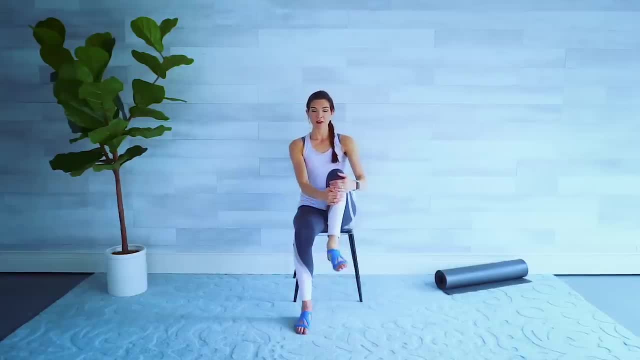 big to the outside. you can also hold your leg here if that's comfortable. reverse the direction of those ankle circles. now let's take that leg, crossing that ankle above the left knee, sitting up nice and tall. immediately you should feel that in your hip and in your glute. if this is, 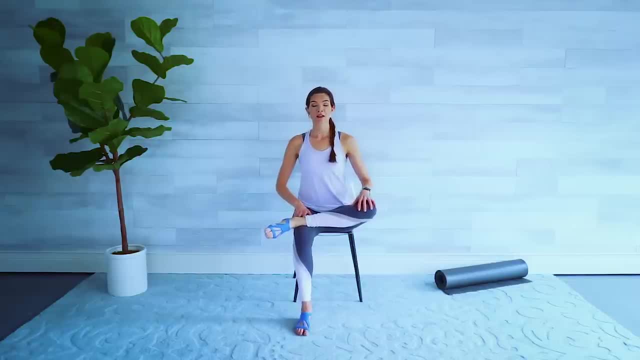 good for you. leave it here. if you'd like to intensify, you can bend slightly over hinging at the hips. this is my favorite stretch, so good for any lower back pain, sciatica issues. hold that there. let's come up again. inhale, exhale slightly over, leaving from the chest. 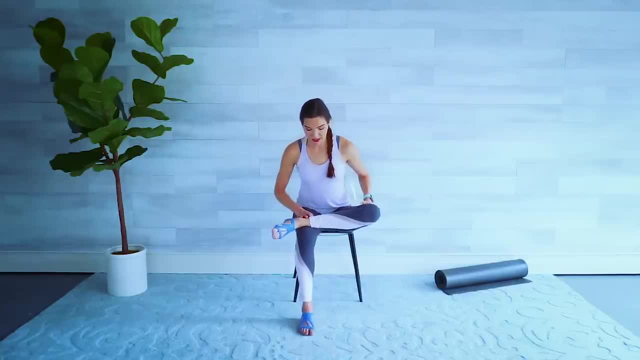 while we're here, we're gonna take that leg, we're gonna drop it, crossing it, sit like it cross-legged all the way over the other and then we're gonna forward, fold all the way over. just think: ragdoll, hang here, inhale, exhale. let's roll it up, go ahead and uncross other side picking up that. 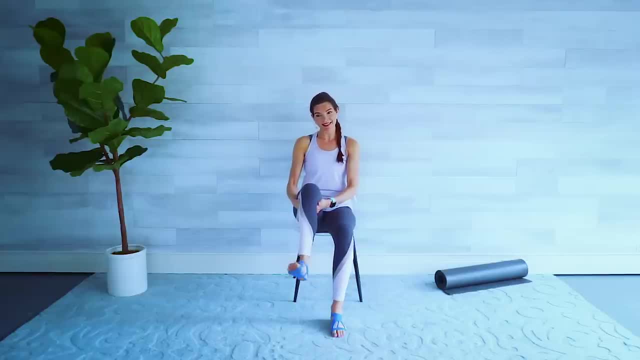 left leg. give me some big ankle circles to the outside and reverse, crossing that ankle over the knee, keeping that foot flexed and then making sure that ankles underneath the knee hinging slightly forward, intensifying that stretch. bring it back up one more time. inhale exhale- bring it back up one more time. inhale exhale- bring it back up one more time. 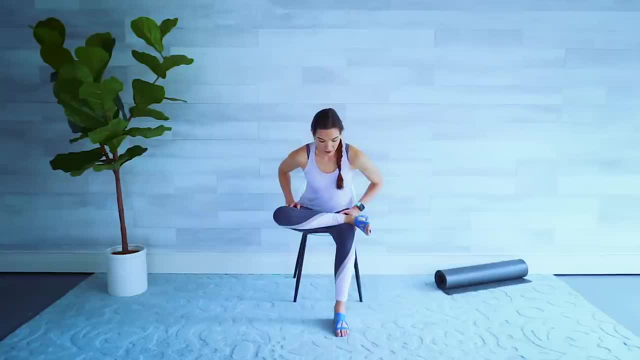 exhale over. I need to scooch that lower leg in a little bit, crossing the legs, and then go ahead, hinge all the way forward, rounding at the back. just hang here, breathe in and out and let's slowly roll it up and uncross those legs. sit up, nice and tall, big, inhale up, exhale, release those arms down. 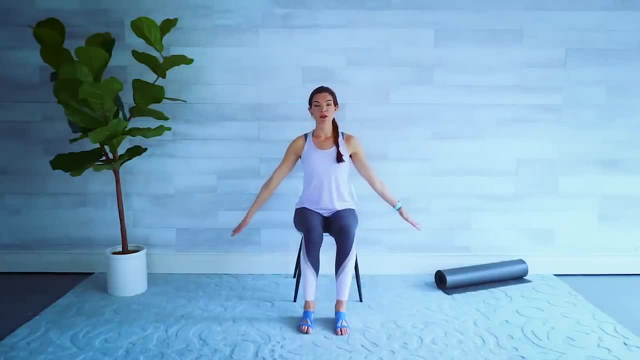 leave them to the sides here, stretching those fingertips all the way towards the floor, really reaching. look over your shoulder, feeling a beautiful stretch in that neck, and while we're here, give me some wrist circles back to center. look over the other shoulder, reversed that wrist circle, mine are popping.